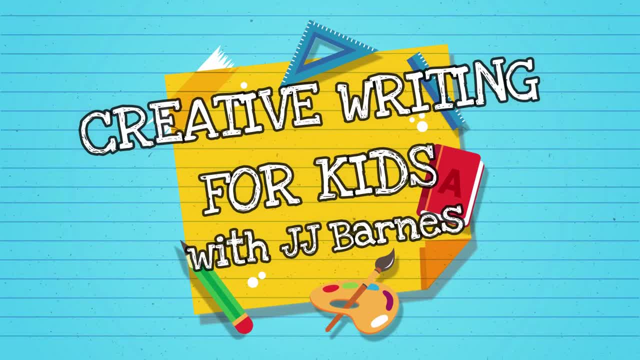 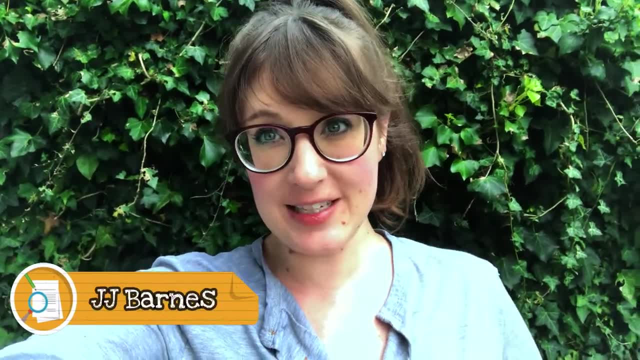 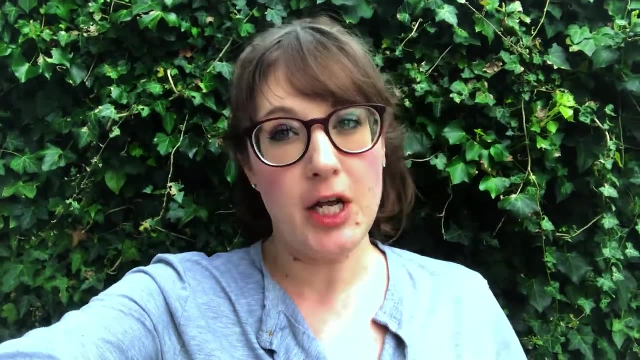 Hi everybody, I'm JJ Barnes and you're back with creative writing for kids. So today I'm going to be doing another writing prompt video with you. I'll be giving you the writing prompt, which I'll also post to my Facebook page, and then in this video I'm going to be talking through with you. 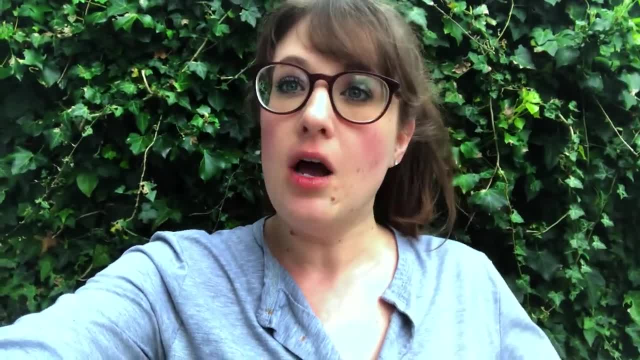 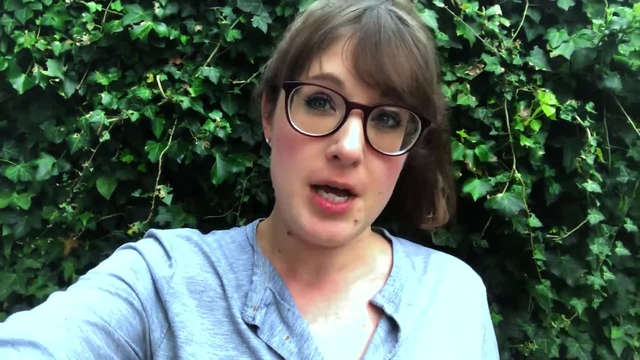 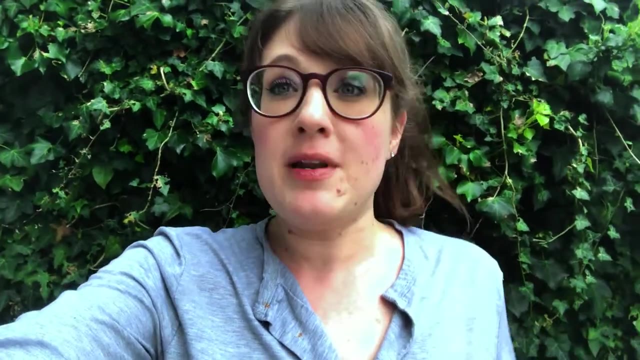 how to think about the writing prompt, what it means, where you can let your mind go and what to do with it. because writing prompts are pretty cool, because if you give a hundred people the same writing prompt, you'll get a hundred different stories because everybody's brain is so different. 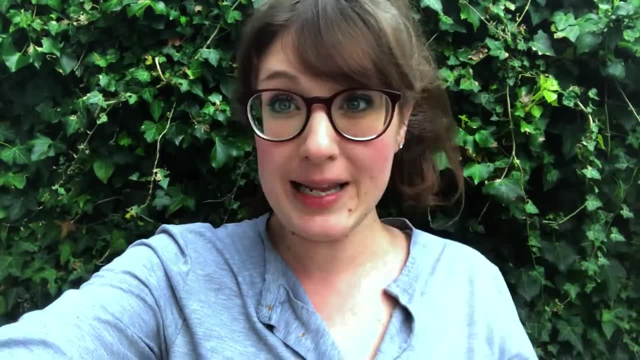 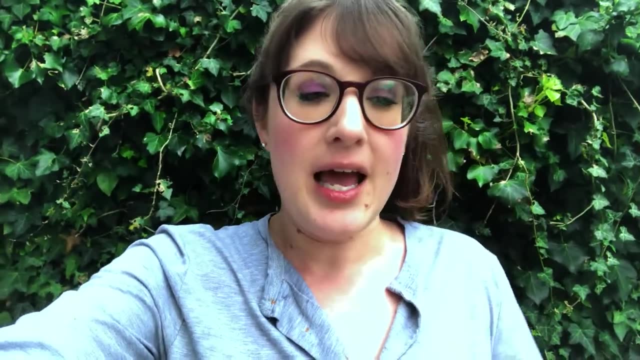 and so unique, and anything you come up with will be completely personal to you. So even if you think it's weird that you're giving the same idea to somebody, it's not because it is just a tiny little seed that you let your imagination run wild. So I'm going to be talking about how to think about. 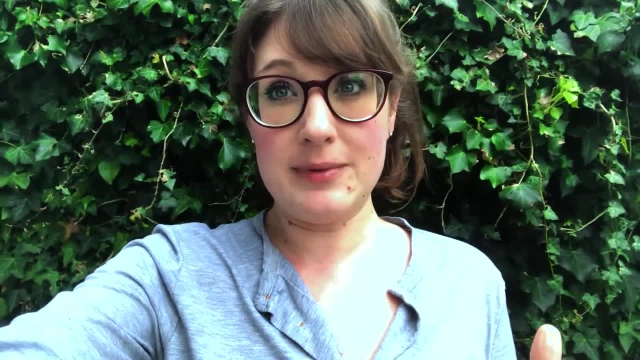 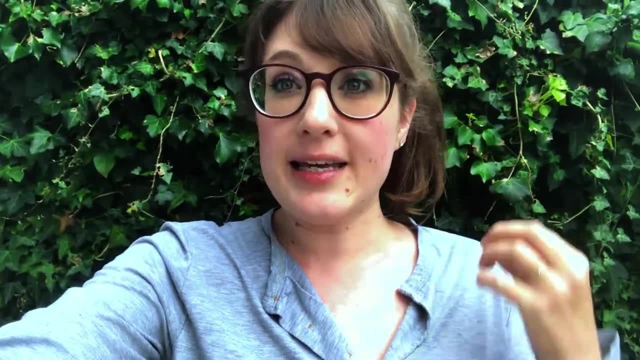 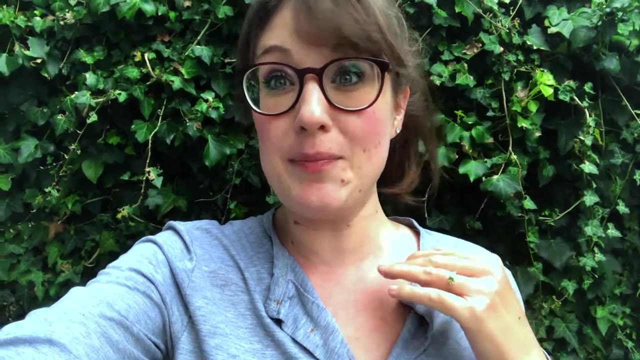 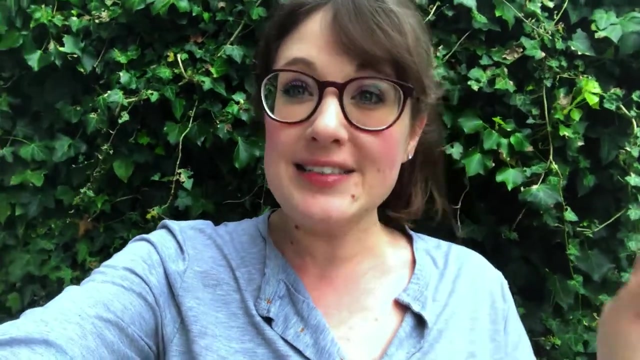 writing prompts and how you can let your imagination then grow. So I really recommend writing prompts if you are looking to get into writing, If you are keen to have a go at writing stories but you're a bit unsure where to start. give these writing prompts a go because I promise you, once you let that story start going, you are going to come up with something that is absolutely, completely unique to you and that is really special and cool. So today's writing prompt: again, I will be posting it online so you can come and show me your stories there. 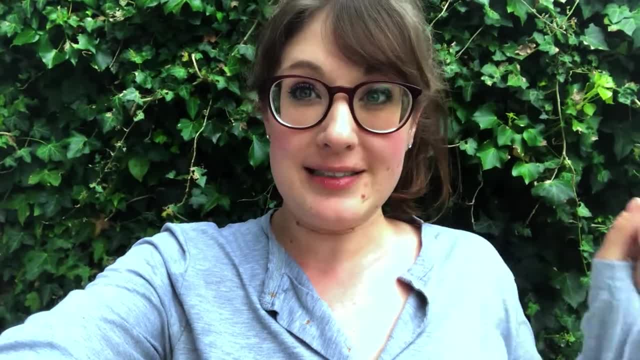 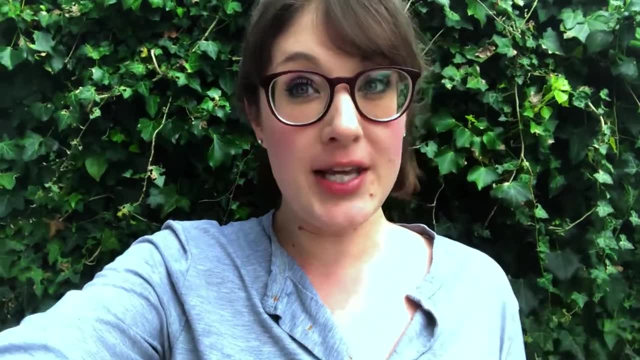 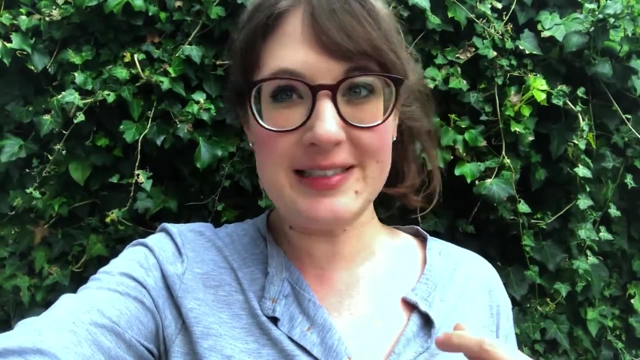 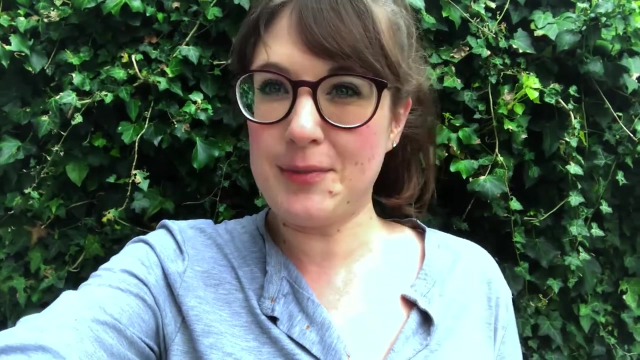 is: you look in the mirror and somebody else is looking back. Okay, so that's your inciting incident: You look in the mirror and somebody else is looking back. So you have to think to yourself: how would you feel? Would you be scared? Would you be excited? Would it be somebody you recognise? Is it a stranger? Is it a monster? Is it someone who looks nice or someone who looks mean? Have you actually been trying to get somebody else to look back? 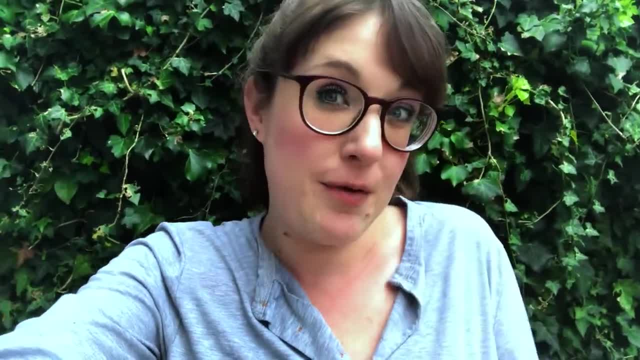 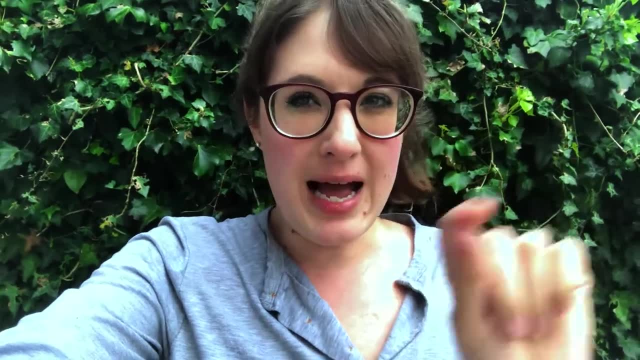 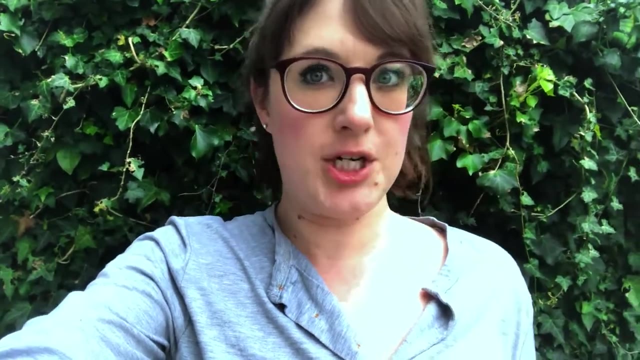 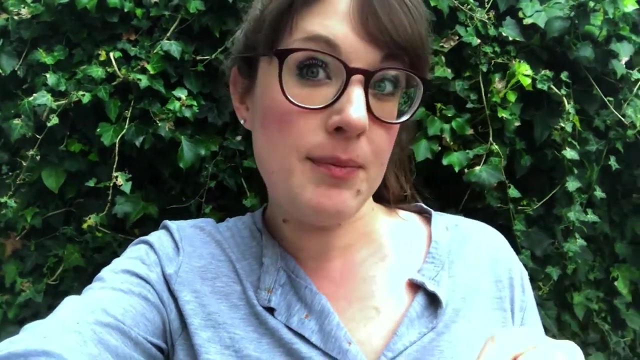 Have you actually been trying to get somebody else in that mirror? Have you done a spell or something? where you're trying to communicate with somebody else? Let your brain start wandering, Okay. and then, when you've had your emotional response, you've felt your feelings and you've worked out that that's somebody else in the mirror. then what do you do? Do you go tell somebody? Do they believe you? Do they think you're crazy? Perhaps you tell the person who has been trying to help you find that person in the mirror. Maybe the person in the mirror 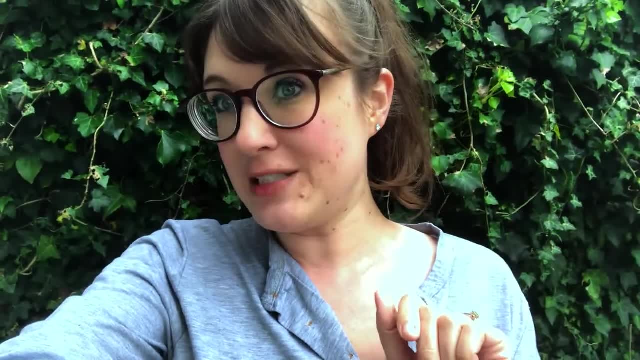 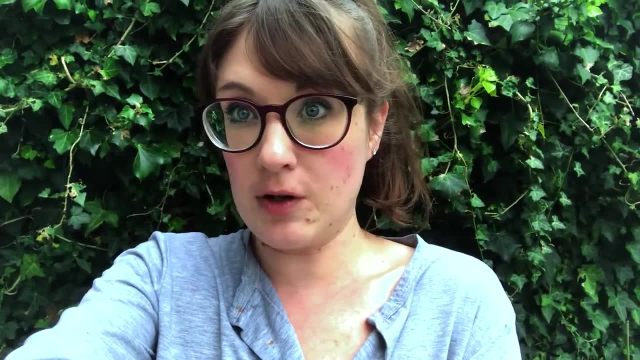 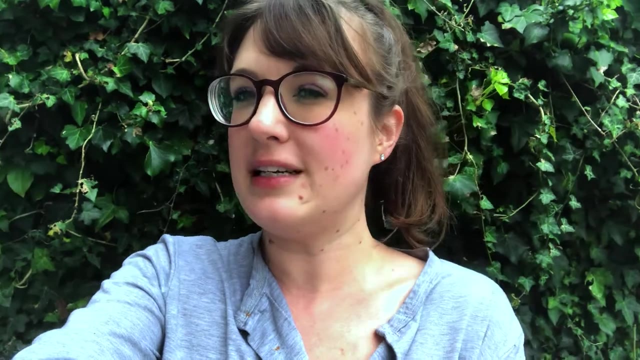 that you've been trying to talk to gives you some information to help you on your quest. perhaps what you've been doing is looking for some mysterious object or looking for somebody who's gone missing, and you know the person in the mirror can help you. okay, do you see what I mean when you start letting your mind wander? 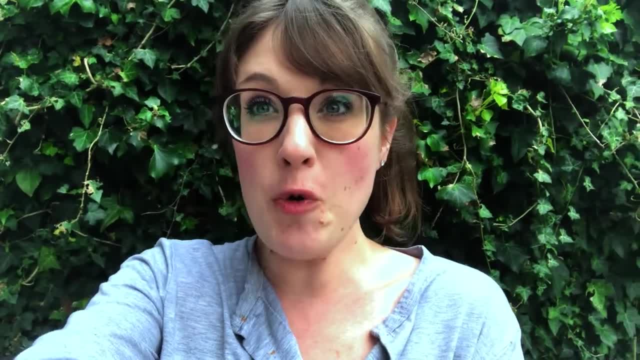 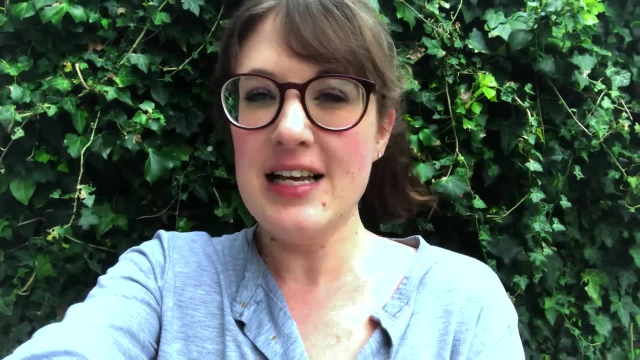 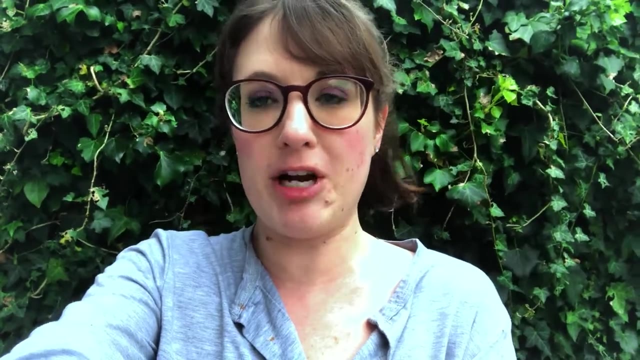 you start exploring that idea. there are so many different places you can go with that story idea and that's pretty exciting. so what you need to do, get a piece of paper or a computer screen or phone, whatever it doesn't really matter. I'm not precious about where you put your stories, as long as you get them. 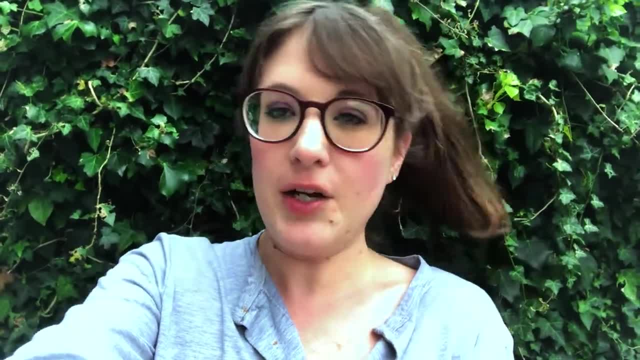 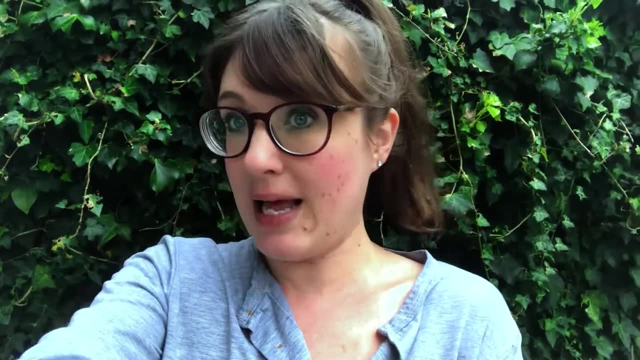 down right, then right at the top, I look in the mirror and somebody else looks back. now what you could do- which a lot of people find really easy, and I find it easy when I'm planning a story- is do a spider diagram. so what you do is you put. 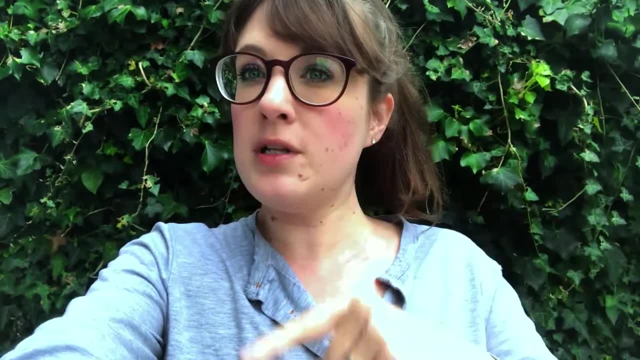 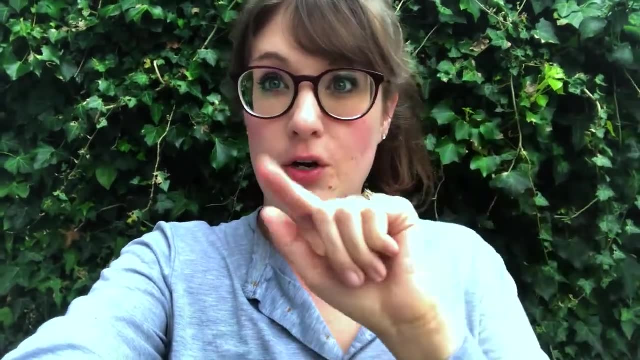 your prompt in the middle and then you put your story in the middle and then you pick your story from the middle of the board and then out of it all the different things that could happen that you want to happen in your story. so how you feel who it is. who do you tell what happens next? what information do you get? 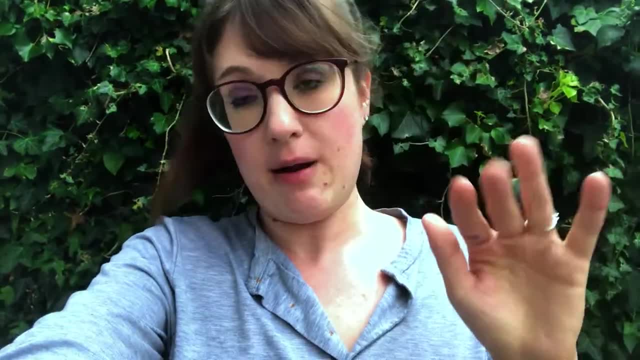 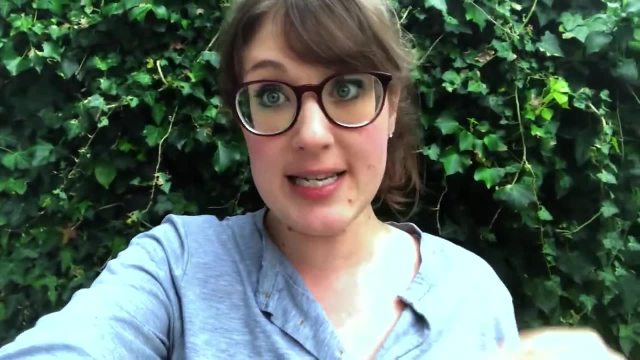 from the person in the mirror, write it all down on a big sheet and then you can start following your diagram when you start telling your story. or maybe you like to do a list, bullet points, things that you have ideas, because as soon as you start writing your ideas down, that's when more come. it's like opening, like a 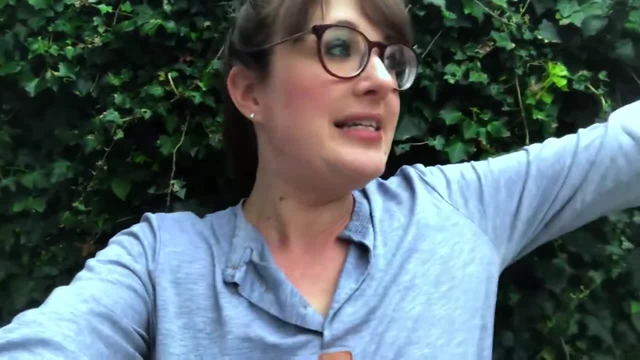 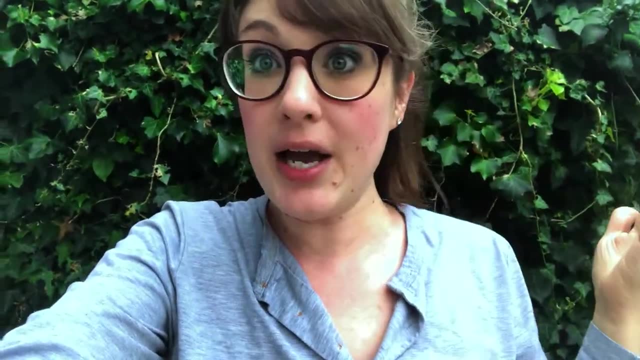 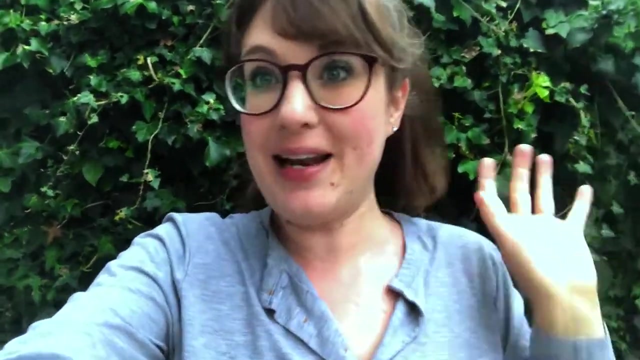 a floodgate and all you lift up your thing and all the ideas start come rushing out and you can start exploring all these incredible thoughts you have in your mind. and it doesn't take much, as long as you start just poking that little thing in your brain, poke it with an idea and then loads.